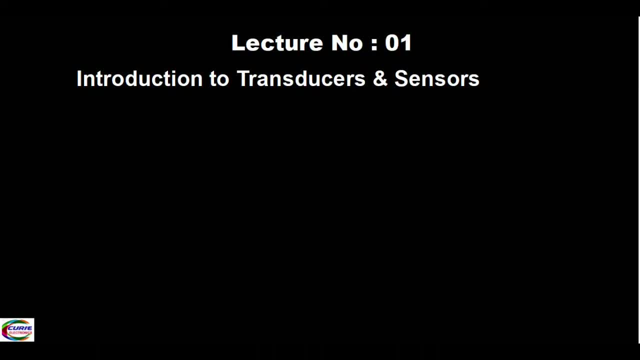 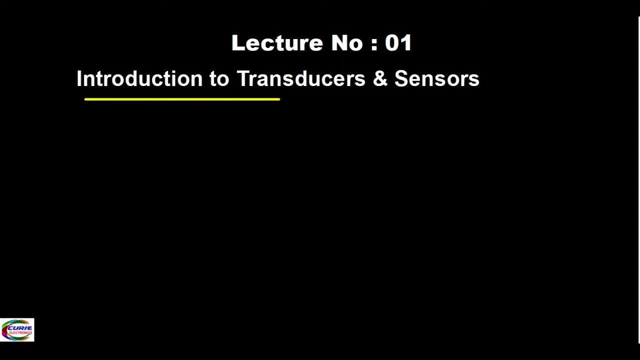 In this video, we are going to learn about transducers and sensors. So what is a transducer? Transducer is a device which converts one form of energy into another form. This is the definition. Transducer is a device that is used to convert. 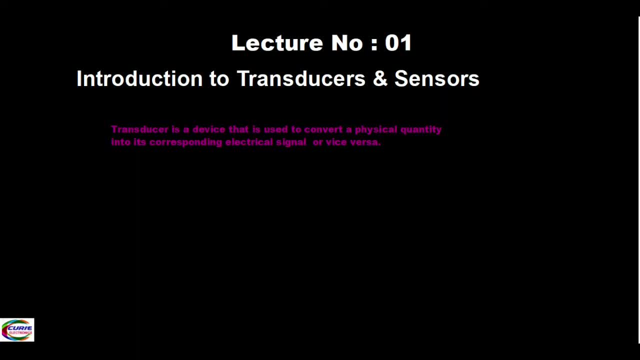 a physical quantity into its corresponding electrical signal, or vice versa. That means if you have a mic, mic acts as an input. This is a voice or a microphone, So our voice will be converted to electrical signal. This mic, electrical signal. This is a transducer. it converts mechanical vibrations to electrical signal. 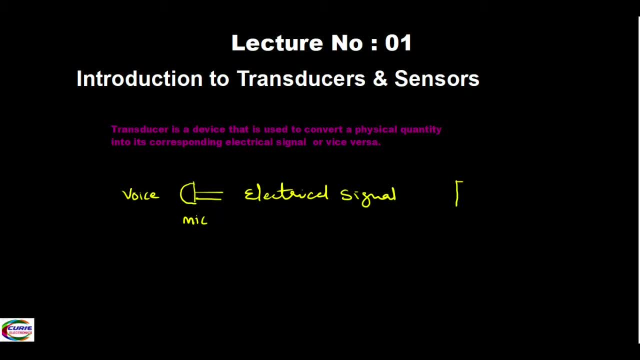 Similarly. or speaker: Speaker is also an electrical signal. Speaker is also an electrical signal. So our speaker is a transducer. It converts mechanical vibrations into electrical signal, a transducer. but it converts electrical energy into sound, sound energy. so transducer, transducer. 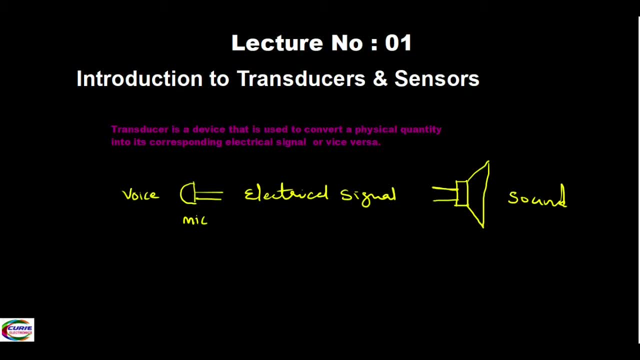 is a device that is used to convert a physical quantity to electrical quantity or electrical quantity to another physical quantity, for that from transfer of energy from one form to another form. that is what transducer then? what is sensor, sensor? this sensors, sensors. the input device that performs an input function- the sensors are almost everywhere- is used as: 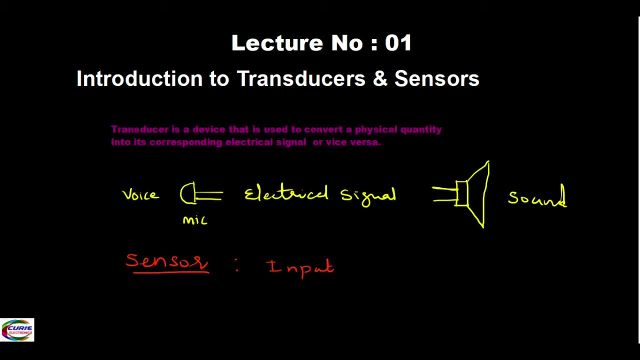 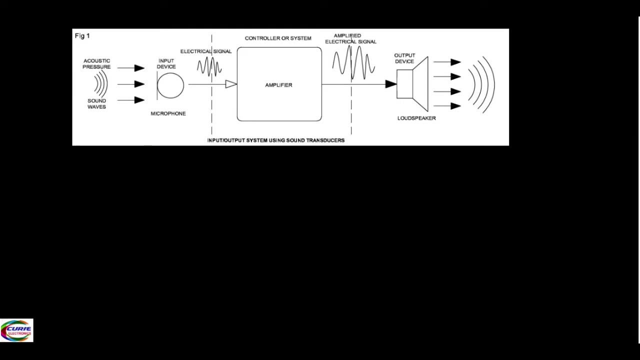 inputs, inputs. so sensor is a device which senses the input. that's what a sensor see in this diagram. you can see sound waves are coming to the microphone- right, it's a microphone- and from there the electrical signal is generated. here this electrical signal is generated, then that goes to the amplifier. 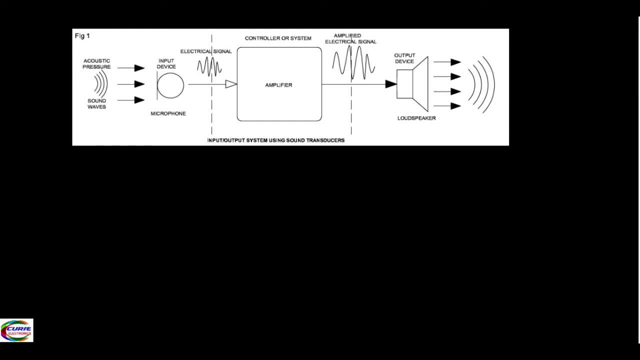 it amplifies and the amplified signal is given to the speaker, so sound is again generated. so this speaker also a transducer, this mic also a transducer. this is mic also transducer. this speaker also transducer. in between is the signal processing, as per our requirement. 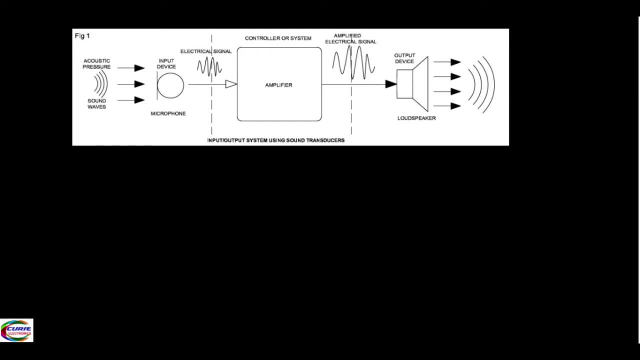 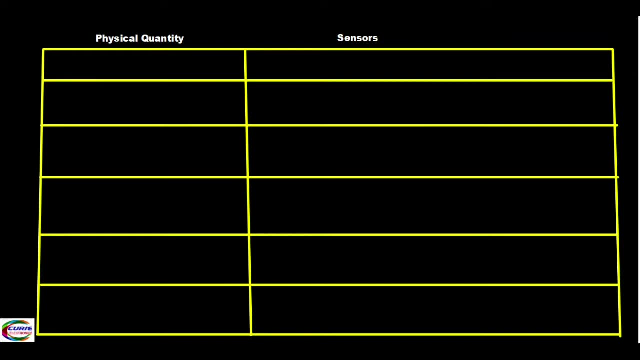 it is not what ribose. it has a verwave mode, so it depends on the user. now we'll see some of the commonly used sensors. now we'll see what is the physical quantity beyond play with, that is light. let light. We have photodiode. these all detect the light. these all say photodiode. 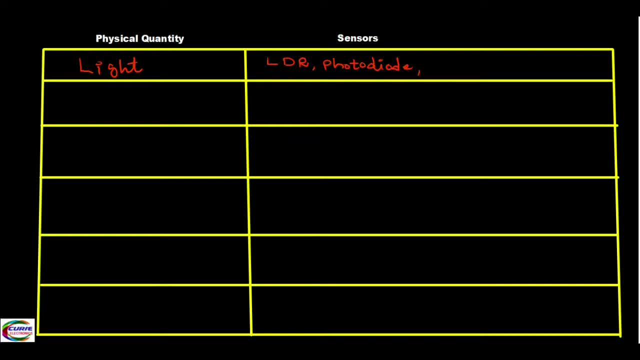 Then what else we have? We have LDR, photodiode, solar cell, solar cell also receive light, solar cell. Then phototransistor, phototransistor, phototransistor. Next, what is other quantity? you tell me which other quantity we measure, that is temperature. 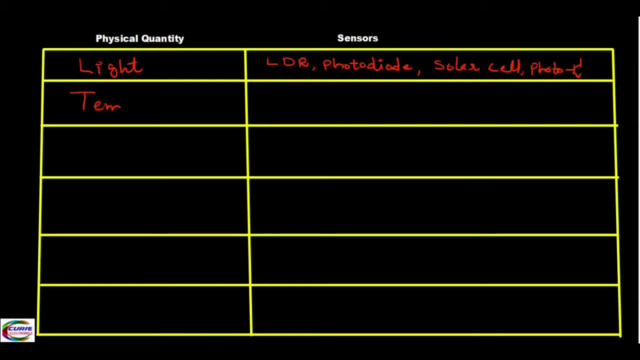 We measure temperature. okay, temperature For temperature. what are the sensors we have? You will say first what you will say: thermocouple. The coming videos we will see what are these sensors, thermocouple. Then one more thing. 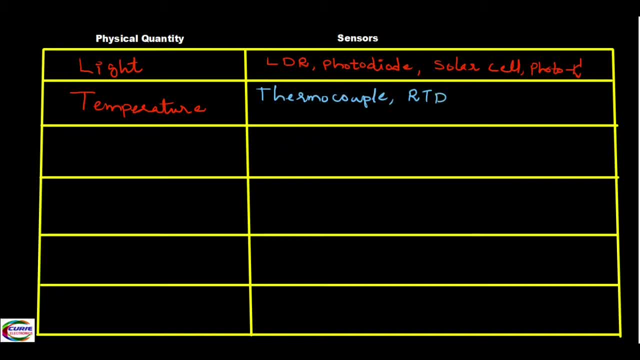 One more device is there: RTD resistance temperature detector. RTD- resistance temperature detector. I will write it here: temperature detector. that is what RTD. Then what else is there to measure temperature? Anything else? Thermistor, thermistor- also a device we use in our electronic circuit- thermistor, thermistor. 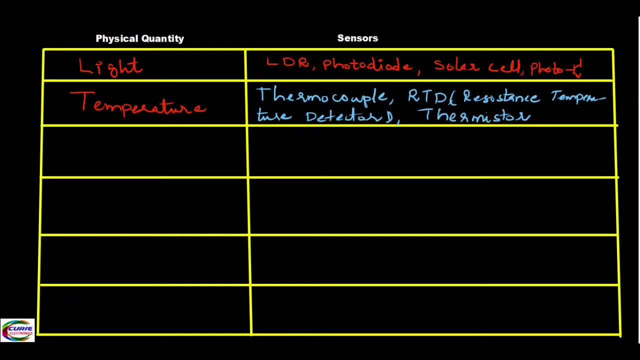 Then light temperature. Then we have another quantity that is also force, force or pressure, right force or pressure. This also we need to sense and to measurement and all we will use. Okay, Okay, Okay, Okay, Okay, This, we will see this. 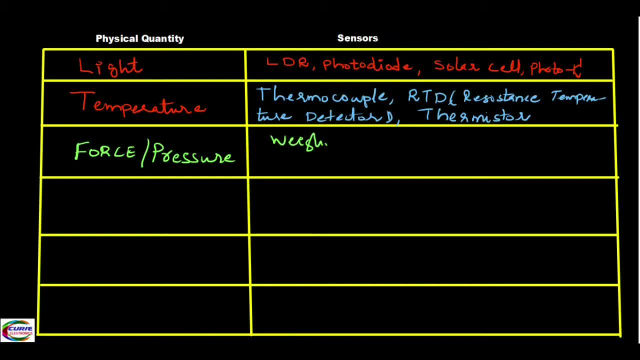 Yes, force. Have you seen weighing scale? This is one of the applications: Weigh scale, Weigh scale, actually what is used in weighing scale? Load cells, load cell, Load cell- That load cell is the sensor. Then we have the strain gauge. 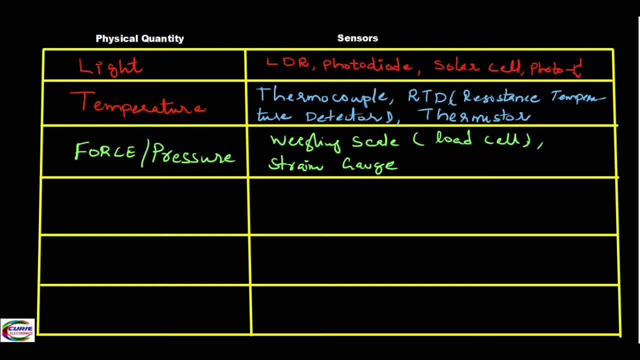 Strain gauge. an idea about the. what are the available sensors stay engaged. uh, there is one more. one more is there that is a pressure switch, pressure switch, pressure switch. okay, now we will see what is the other thing: light temperature force, then position. position, also an. 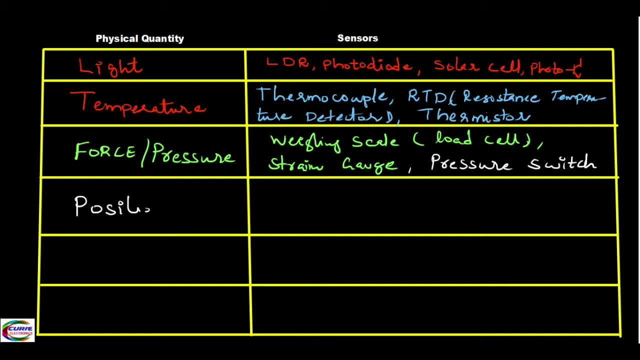 important quantity we have to measure in automation. and all so for the position we use potentiometer. potentiometer, that's a variable resistor. it rotates from that rotation we will get the idea, then encoder the washing machine panel and all one rotating knob will be there. 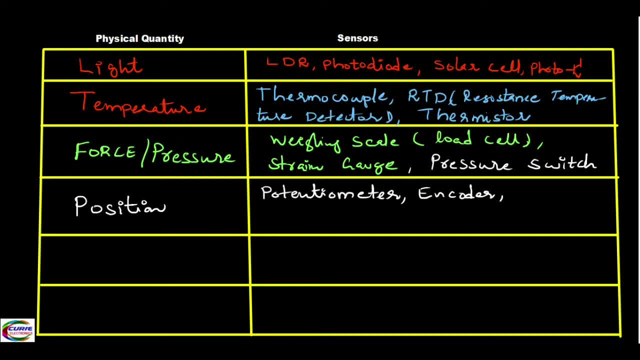 that is actually encoder, and then lvdt, linear variable differential transformer, lvdt. okay, these are the popular ones. then again, what we have after position? what is the quantity speed, speed also, we have to measure and process many times those that one of the sensor is tacho generator. 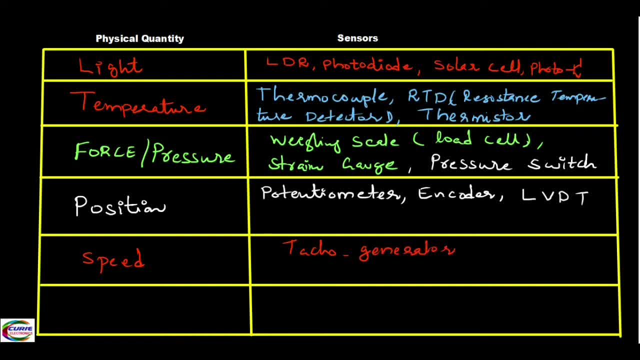 this is used with the motors: what speed motor is rotating to find. so the sensor name is tacho generator, then the traffic light, traffic signal and if we jump, there is a sensor to find that is a doppler based sensor, doppler doppler sensor. this also measures speed, doppler sensor. and